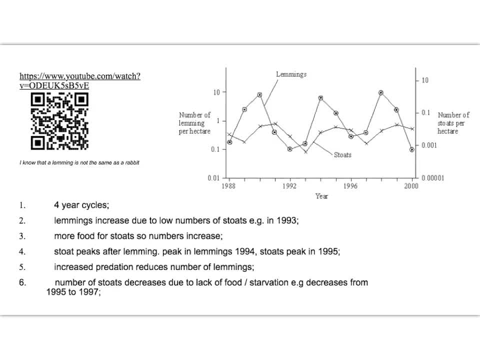 We'll see an example in the next page. So here we've got the stoats and lemmings. So stoats the predator, lemmings the prey. There's a nice video to watch here. It's about rabbits and stoats, but it illustrates the point. 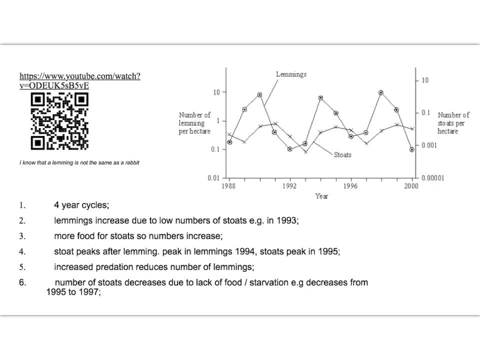 So let's look at the framework and apply it to this question. So it's a four year cycle and you can see that the difference between the peaks or the troughs, is about four years. If you look at the peak here, that would be 1990.. 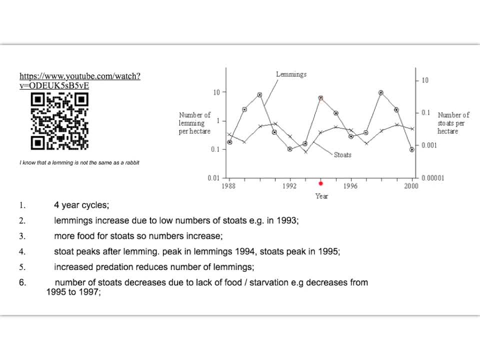 If you look in the peak here for lemmings there that would be 1994.. So four years. So first of all, and you can start anywhere within the cycle, really, unless this directs you in the question. So we're going to start that. lemmings increased due to low numbers of stoats in 1993.. 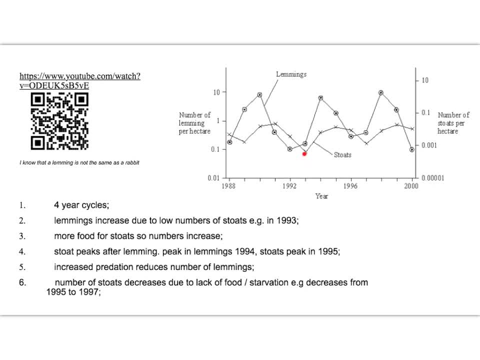 So you can see here a trough in stoats. so very low numbers. You can see at that point the lemmings start to increase. after that That's good. Then, as the lemmings start to increase, there's more food. 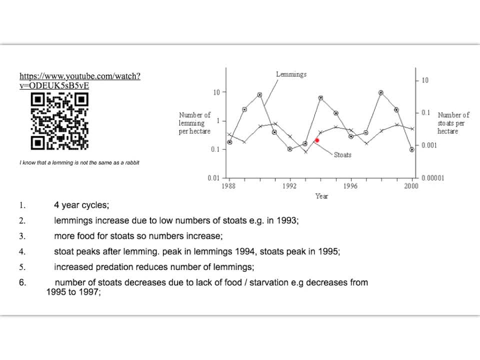 There's more foods for stoats, so they start to increase And you can see that here as they're increasing, later on the stoats will start to increase. The stoat peaks after the lemming, So the predator is peaking after the prey. 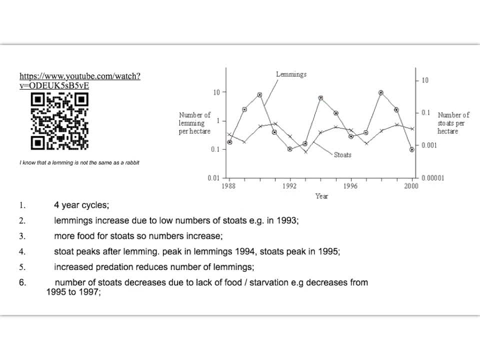 So the peak in lemmings in 1994.. And then after that you get a peak in stoats in 1995.. You've then got now here in the graph. you've got increased predation, And so you get a reduction in the number of lemmings.